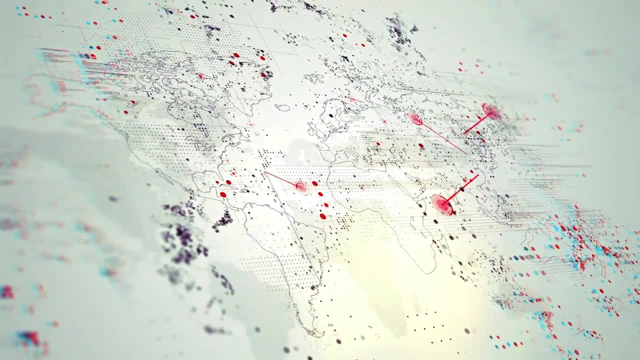 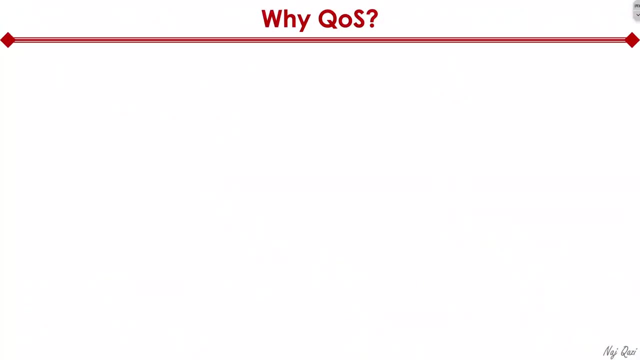 Now let's shift our attention to QoS. Before I get into the mechanics of QoS, let's ask ourselves the question: why? Whenever you learn a new piece of technology, it's crucial to take a step back and ask yourself: why does? 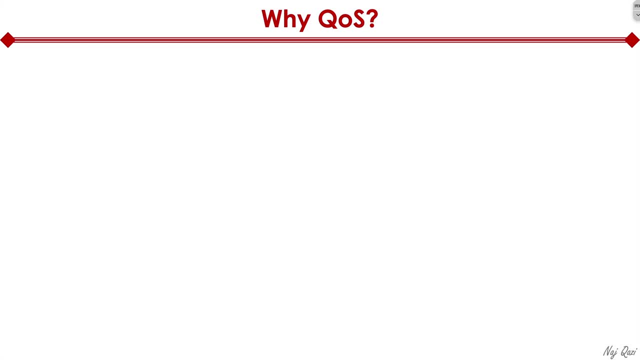 this technology exist? What problems is this technology designed to solve? If you make this a habit, I promise you your level of understanding will be completely transformed. With that, let's jump into why QoS First. QoS stands for quality of service. Here I've got a very small. 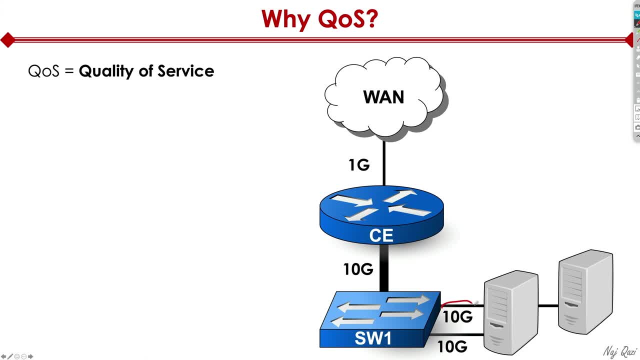 network and what I have in that network is two servers each connecting at a 10 gig level. So I've got potentially 20 gig worth of capacity being utilized from downlink's perspective. But if you look at the uplink, the uplink on the switch is limited to 10 gig. 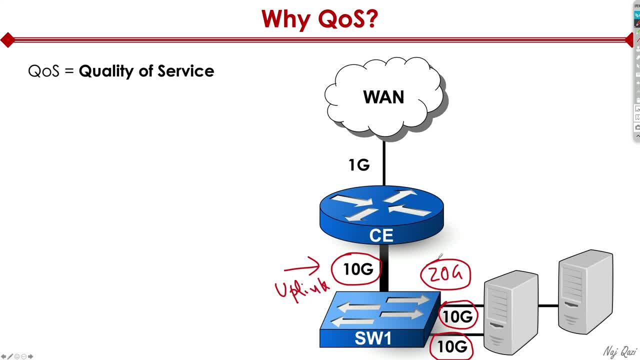 So that's a two to one speed mismatch. And then when we go from the switch to the router, the WAN circuit that we have is one gig. So that's actually a 10x mismatch. So, as you can see, as we continue going upstream in our network, we have more choke points. 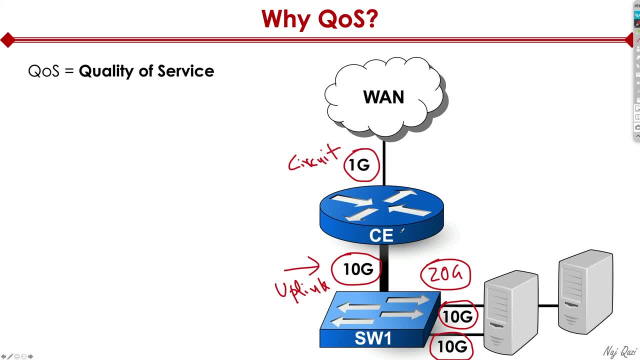 And the speed mismatch causes packets to sit in the buffer, which is a place in memory, And traffic just sits there until it's processed. And what causes traffic to sit in the buffer? If way more traffic is coming in into the device, then its ability to be able to deliver traffic on its outbound interface. 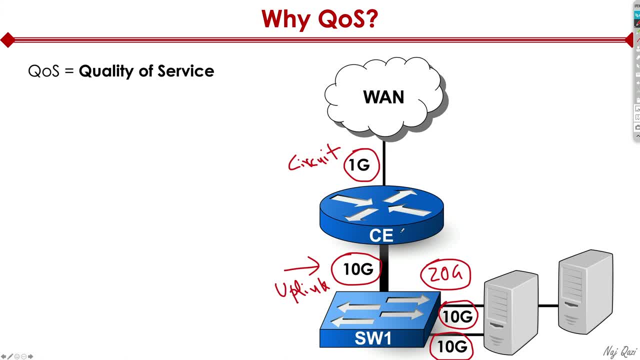 then that traffic has to be queued somewhere, It has to sit in a buffer somewhere, And that's where QoS comes in. As I just finished talking about, these are the two network choke points: the uplink from the switch into the CE. 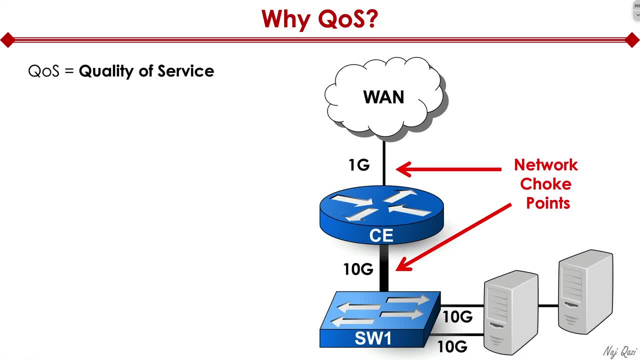 or the customer edge router and the WAN circuit that is terminating on our CE. Now here are today's network challenges. So if you think about your voice flow, for example, if you happen to be on a zoom call or Skype or Microsoft Teams or WebEx, 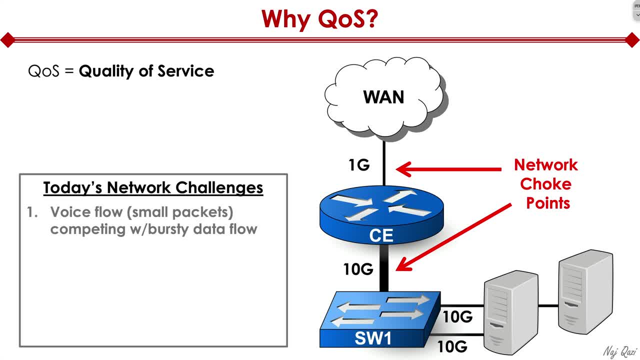 your voice packets are very small. Contrast that to somebody who's on YouTube watching a 4k video or ultra high definition video. it's going to absolutely crush your voice flow And that's not a good thing. That's a terrible thing. There is a way to manage that. 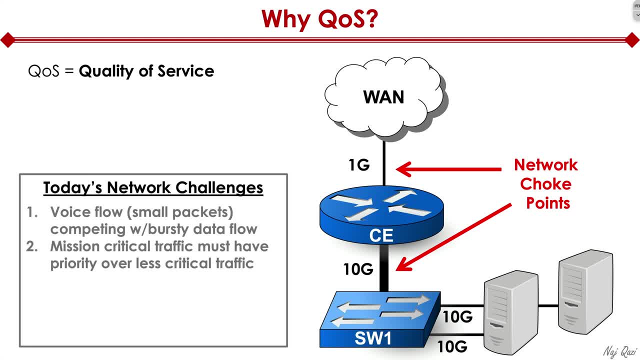 but it is. It's a challenge that we have to look into. Also, your business mission: critical traffic must be prioritized over less critical traffic. So if you happen to be a retail shop, definitely the credit card swipe is the most critical traffic to your business. that has to be prioritized over guest. 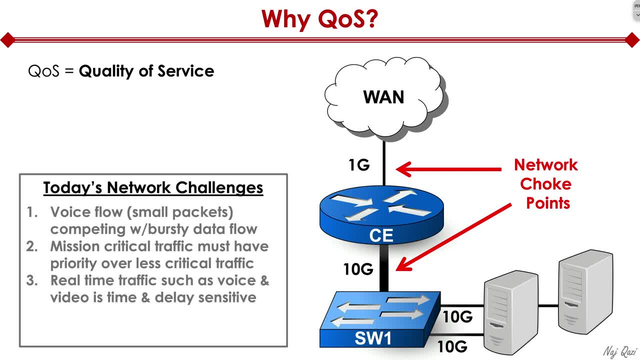 wifi, for example. Also, the real time traffic, such as voice and video, is time and delay sensitive. I'll talk more about the real time traffic in a bit. And finally, in today's network, the expectation is that there's going to be zero downtime network that's always available all the time. 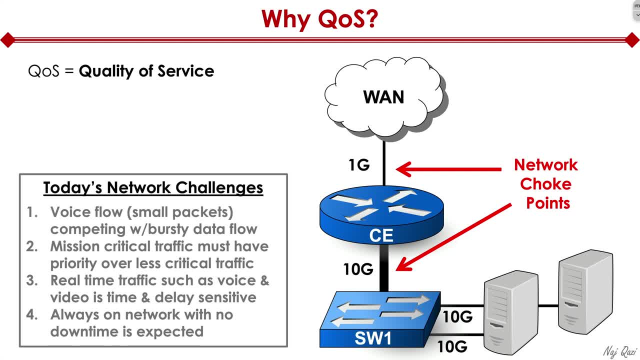 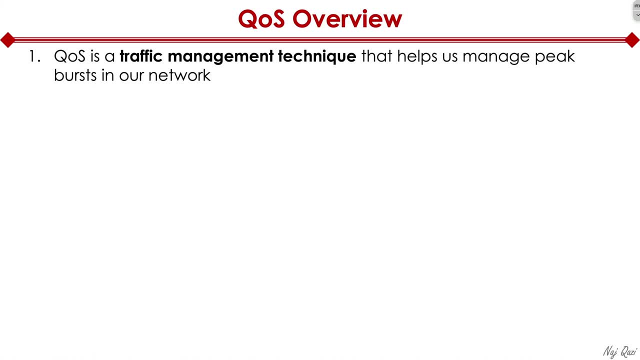 like any other utility, like water or power. Now, that said, let me give you a quick overview of QoS. So, hopefully, up until this point, I've built a business case for you to understand that we need traffic management technique. And that's exactly what QoS is, because when we have a traffic mismatch or choke points in our network, 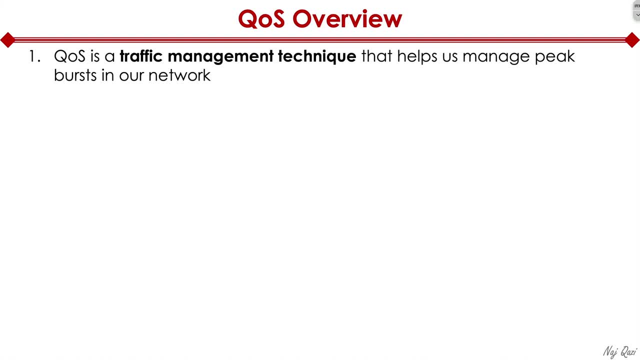 that traffic has to be dealt with, And that's where QoS comes in. It helps us manage peak bursts in our network. Now, one key thing I want you guys to keep in mind is if your network is congested all the time. 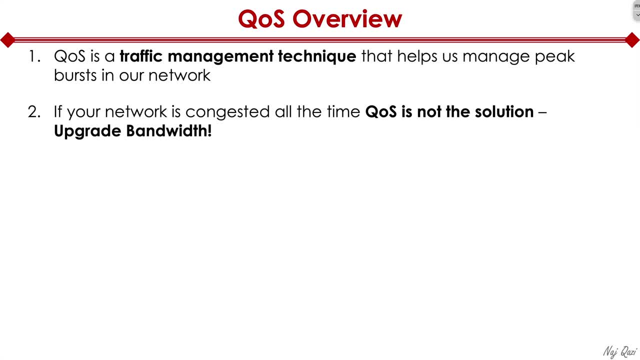 QoS is not going to solve your issue. You absolutely need to upgrade your bandwidth. QoS will only come to rescue if your network is congested at certain times of the day, For example, first thing in the morning when people walk into the office. 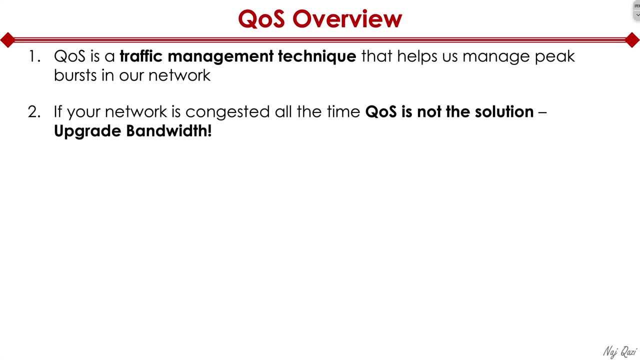 the login. you're going to see a little peak there. Also certain times of the day when there are certain activities that get kicked off, like some sort of backup, that can be managed with QoS, But if your network is congested all the time, 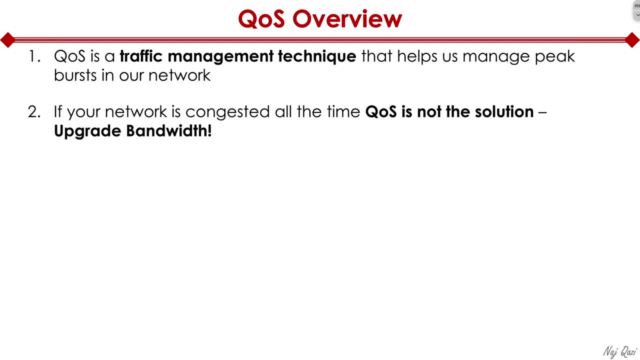 you have bigger issues, You absolutely need to upgrade your bandwidth. The whole idea of QoS is to provide unfair advantage, as I like to call it, to certain types of traffic on our network, And naturally, you might be asking yourself a question. 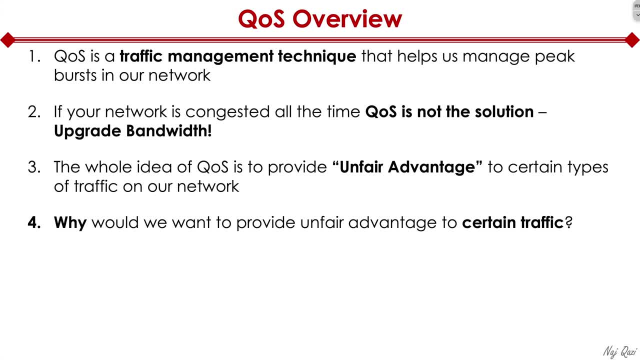 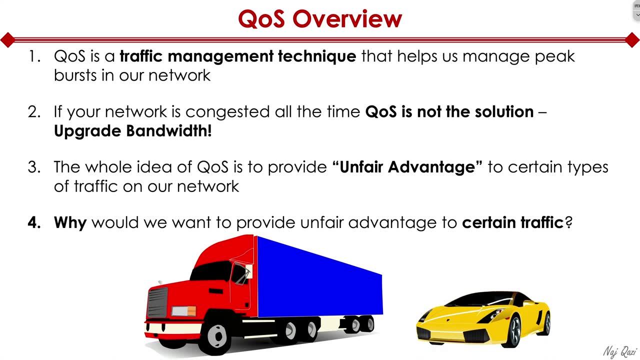 Why would we want to provide unfair advantage to certain traffic? Well, let me give you an analogy. So if you have a 10 wheeler truck like the one you're looking at, and then you have a beautiful Lamborghini right behind that 10 wheeler, 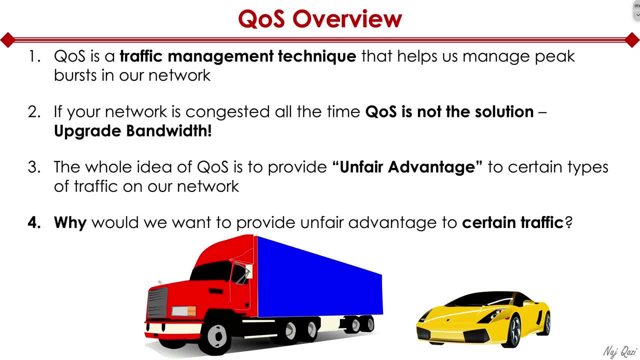 Well, the Lamborghini could go 200 miles an hour, whereas that truck might only go up to 80 miles an hour. Well, we got an issue. Plus, the truck is much bigger and it- and let's imagine if it's- a single lane road. 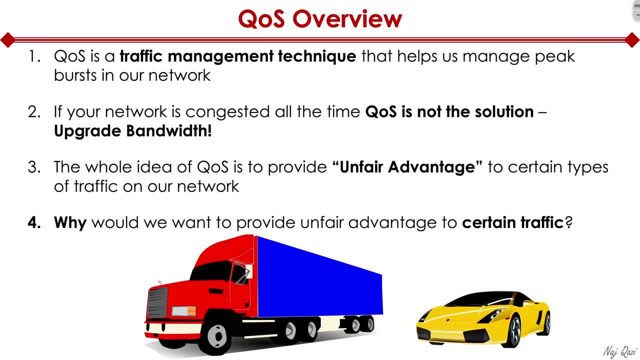 Lamborghini is going to be stuck behind that truck for a while until we get out of the one lane situation. So in our network what we do is we create unfair advantage for certain types of traffic, which in this case is a Lamborghini, to allow it to have priority so it can actually get past the truck because it can move faster. 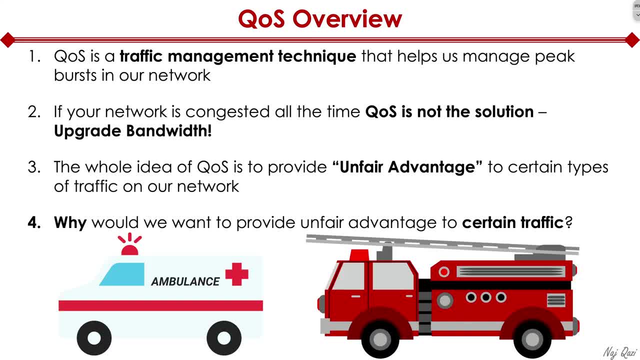 Other examples could be like ambulances, ambulances and firetrucks having the ability to use emergency lanes to be able to provide services to the community. So we're in a sense providing an unfair advantage to them so they can provide better service to the community. 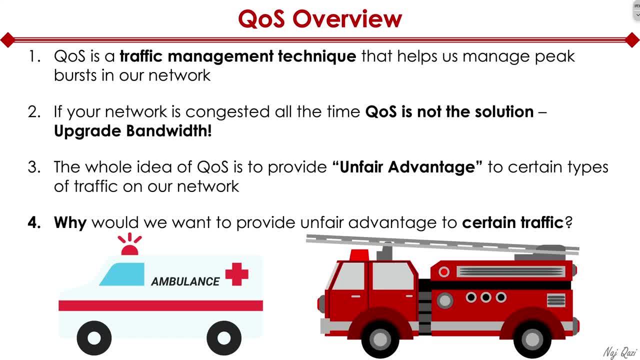 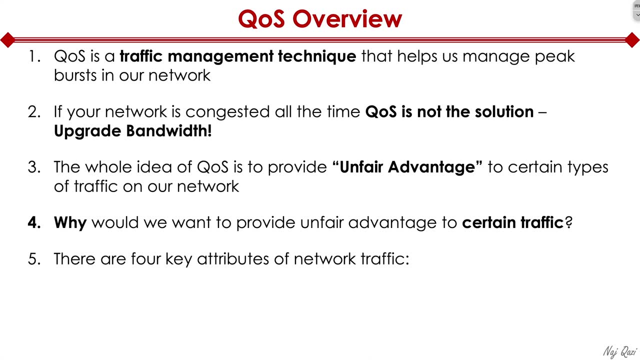 Similarly, in QoS, we have the ability to allow certain type of traffic to be able to provide better customer experience to our users, And there are four key attributes Of network traffic that we must absolutely know about, and we have to know them cold to understand and master QoS. 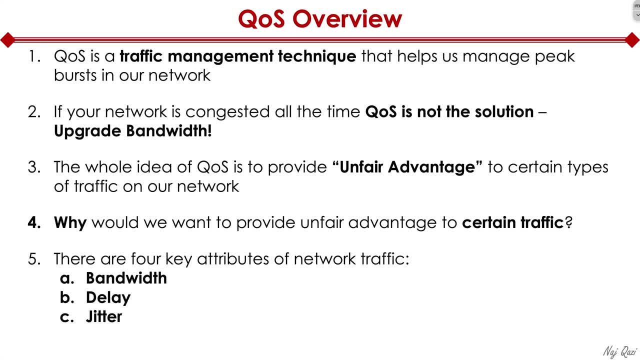 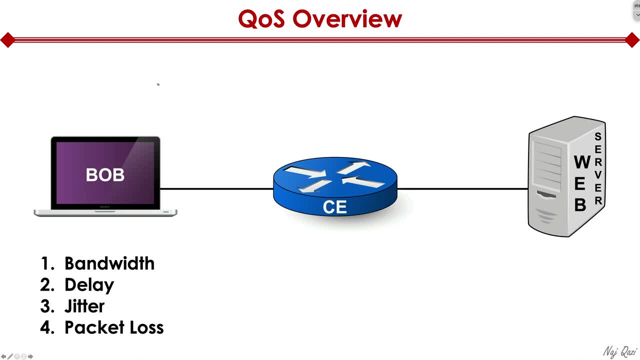 First is bandwidth, Second is delay, Third is jitter And fourth is packet loss. Now let me dig deep into each. So what's the bandwidth? now, Bandwidth is the speed or capacity of the interface in bits per second. So, for example, 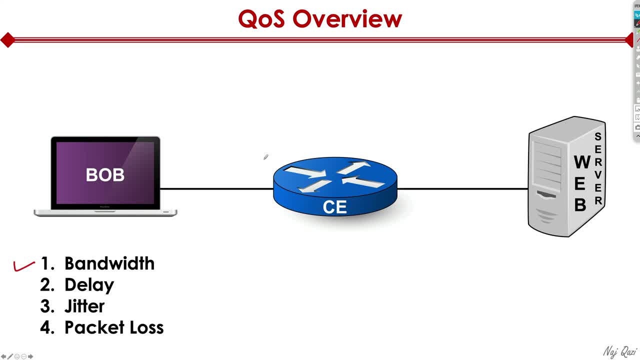 Bob's laptop might be connected Into this customer edge router at one gig and the other interface on the CE might be plugged into the web server at 100 meg. Now, as you can see, there is a 10 to 1 mismatch when it comes to bandwidth or speed. 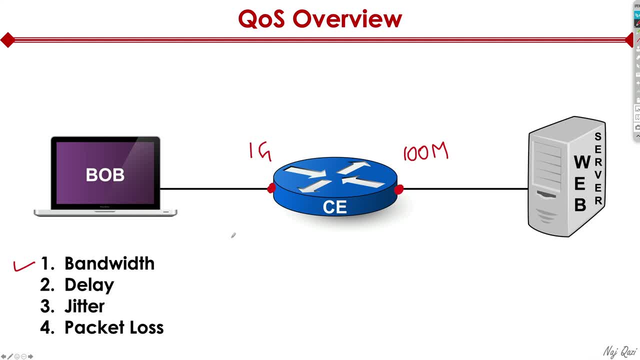 So what this would do is the laptop will have the ability to send a lot more traffic into the CE. Then the CE is capable of forwarding over to the web server. Now this web server might have different types of traffic. It may have, of course, the web traffic, and it may also serve some other. if it's a unified server, it might have the ability to process voice and video. 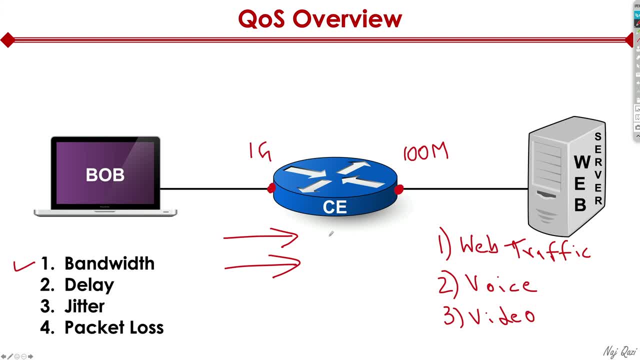 So, to deal with this traffic mismatch and to do this efficiently, what the router would do is it would create different queues. Okay, so it will create, let's say, QA, it will create QB, so on and so forth, and it might say that, hey. 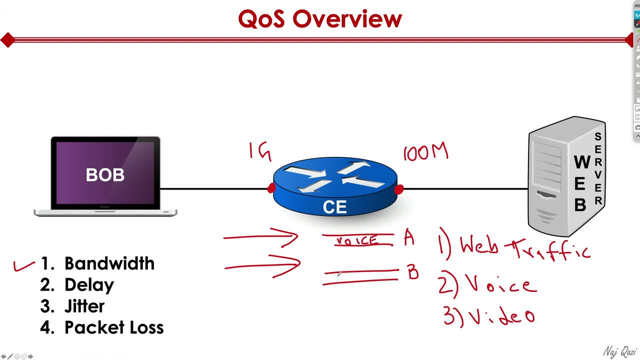 Okay, so it will create, let's say, QA, it will create QB, so on and so forth. All the voice traffic can be put into QA and all the data traffic could be put into QB, and the voice traffic will get a high priority over the data traffic, because the data traffic can be dropped. 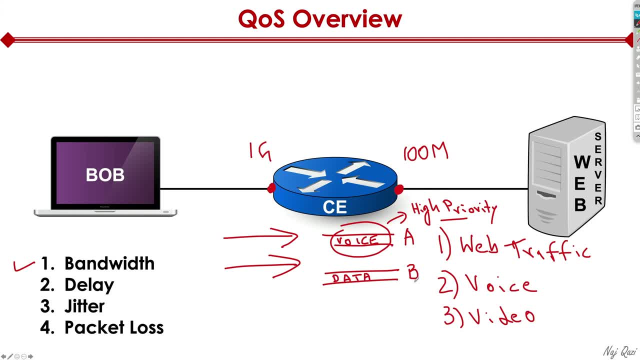 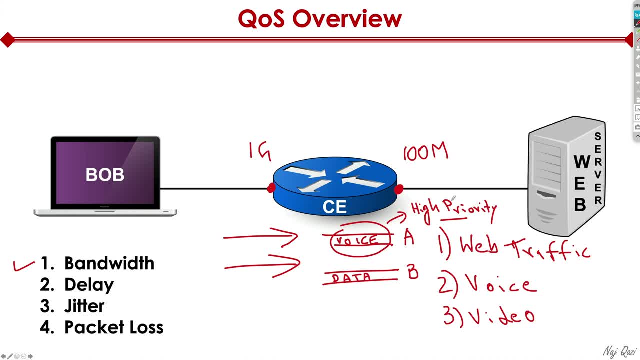 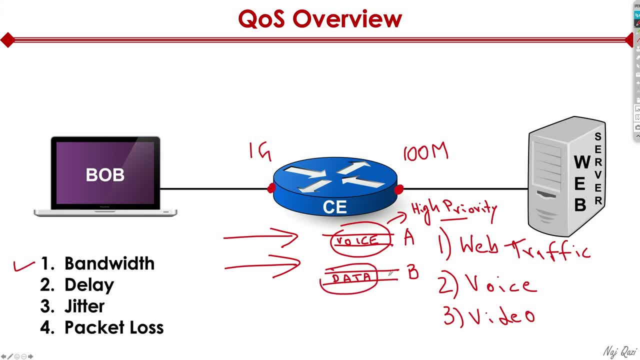 So this is a very high level, rudimentary example, but I'll dig a lot deeper as we continue moving forward. The next thing I want to talk about is delay. Delay is the time it takes for a packet to travel from source to destination. 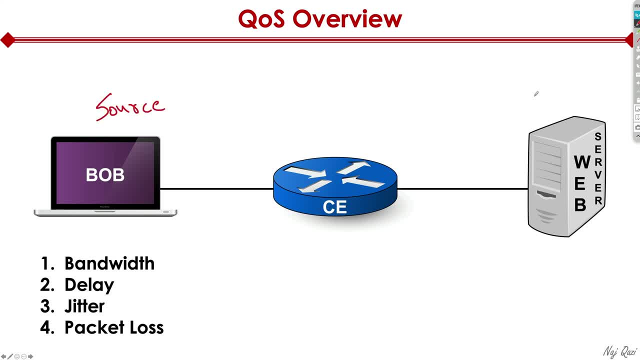 So Bob Could be the source and web server could be the destination. It's the amount of time it takes for the packet to travel, and that's what we call a one way delay, because that's how long it takes for packet to go from Bob's laptop to the web server. 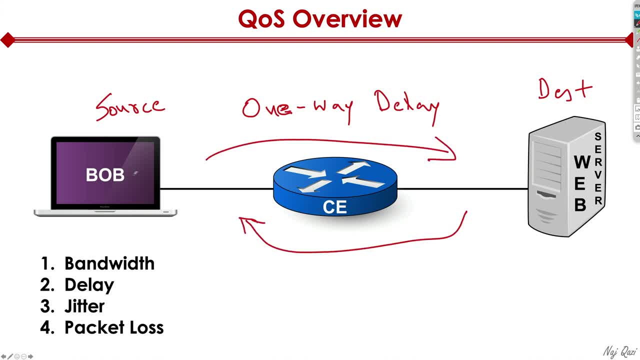 But if you were to measure traffic in both directions, for that flow, to go from Bob to the web server and then come back around that entire thing? It's called round trip delay, because what we're capturing now is the amount of time it takes for the packet to go back and forth. 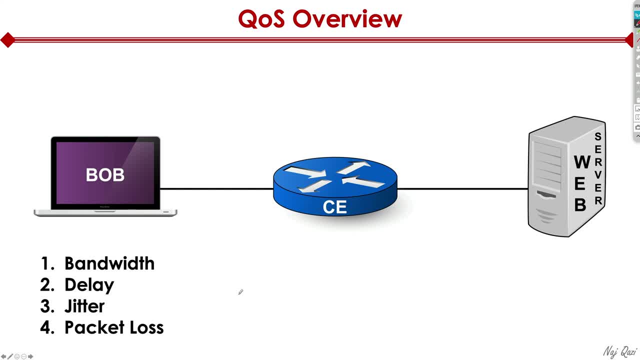 The third element here is jitter. Now jitter is a variation in one way: delay between continuous packets or a packet flow. So, for example, Bob may send multiple packets. So let's say the first packet sent experiences a latency of 100 milliseconds. 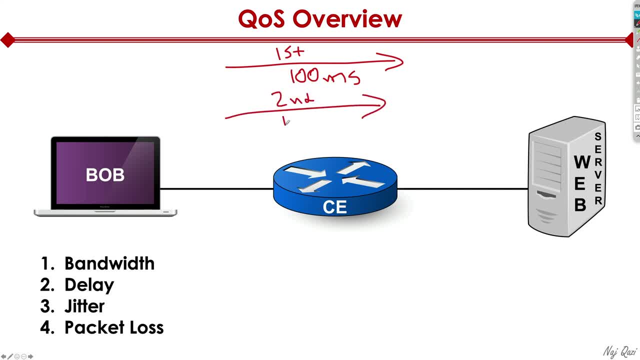 The second packet may experience a latency of 120 milliseconds And then the third packet sent may experience a latency of 150 milliseconds. So, as you can see, between the first and second packet we have a discrepancy of 20 milliseconds or delay of 20 milliseconds. 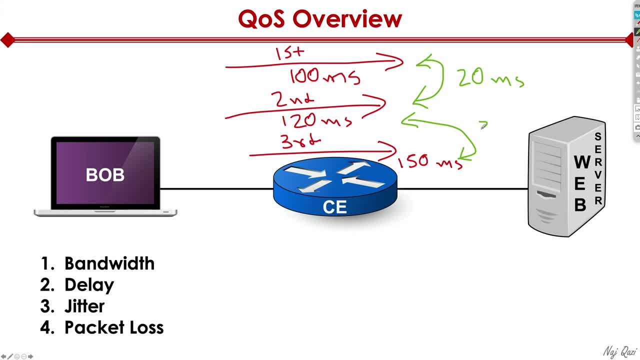 And between the second and the third packet we have a delay of 30 milliseconds. This difference in delay And delay is called jitter, And it's an absolutely terrible thing, especially for voice and video, real time traffic And, finally, packet loss. 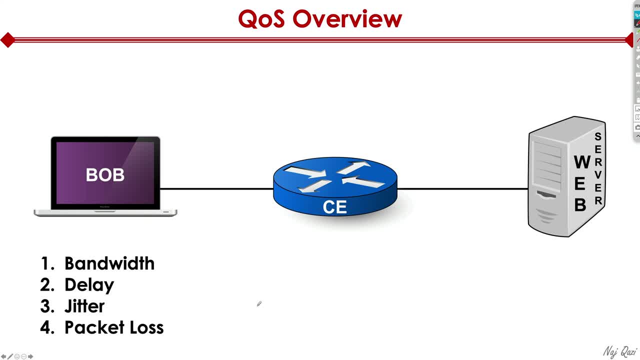 Now, packet loss is the amount of lost packets on an interface, represented as percent of lost packets. So in this example, if Bob sends 10 packets and the web server only gets five, that means we had a 50 percent packet loss And that is terrible. 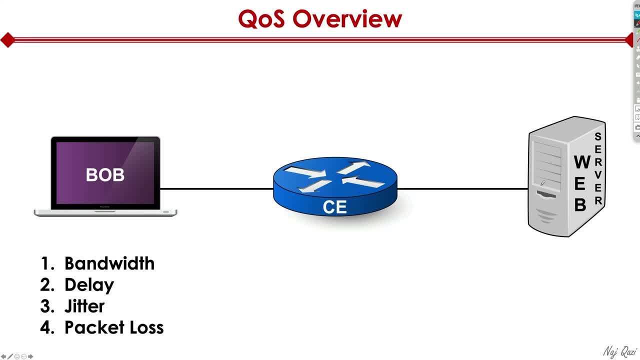 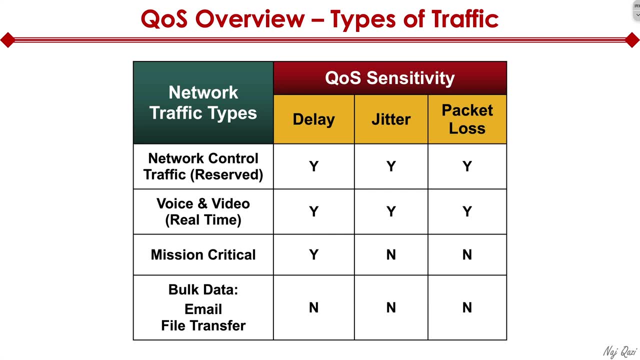 In times of congestion, traffic gets dropped and QoS tools can help us manage that aspect. Now let's talk through different types of traffic. I've got this chart here to show you how different types of traffic in our network is treated and whether or not it's delay and jitter and packet loss sensitive, because that is the most crucial thing to know before we learn the mechanics of QoS. 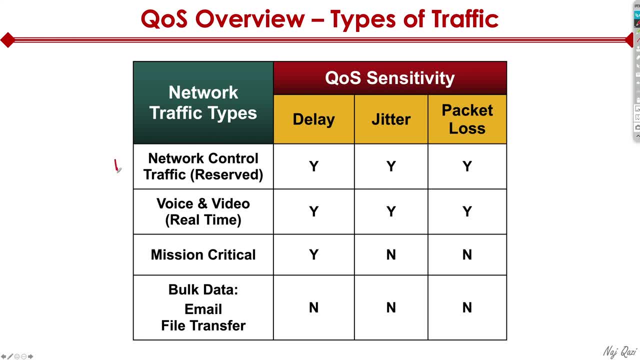 What I have on the left is network Network traffic type. So the first type of traffic that I have here is network control traffic, which is reserved. The second type of traffic is voice and video, That's real time traffic. The third type is mission critical. 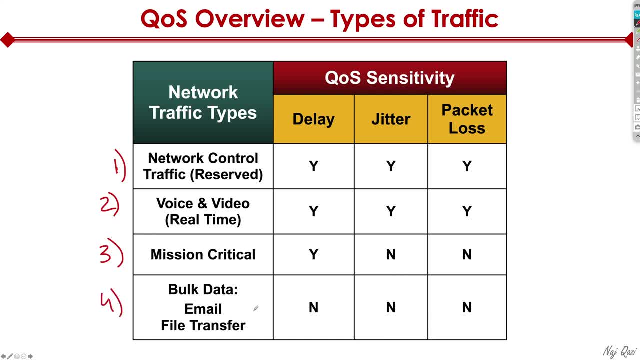 And the fourth type is bulk data, Things like email file transfer. Now the network control traffic is reserved. That is not something we can change or manipulate. Routers and switches automatically prioritize their network control traffic on anything else. When I say network control traffic, what does that mean? 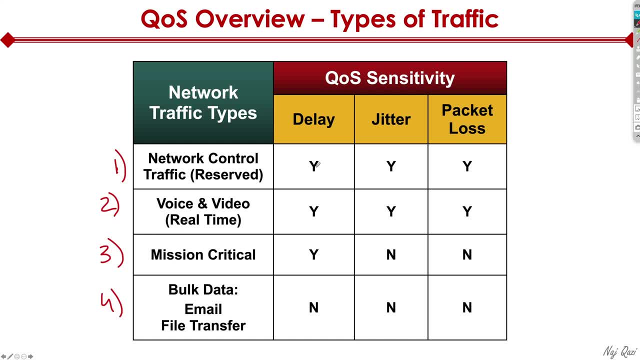 Things like spanning tree at layer Two or OSPF or BGP at layer three or routing protocols, That traffic must be prioritized, because that's what allows switches and routers to build paths and traffic flows, So that path has to be available for the network to continue operating. 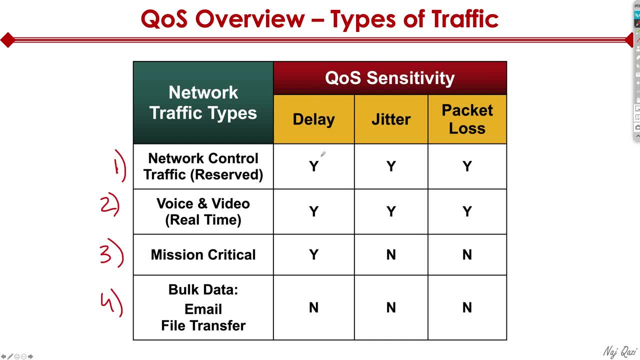 So that is always super prioritized And network control traffic is delay sensitive, jitter sensitive, packet loss sensitive because it absolutely has to function before anything else. Now, voice and video traffic is also delay sensitive, jitter sensitive and packet loss sensitive. The mission critical traffic typically is delay sensitive, may not be jitter sensitive and it may not be packet loss sensitive, especially if it's TCP based. 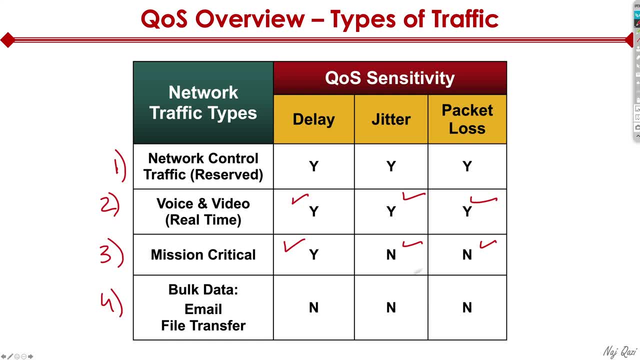 It can always be retransmitted. so it's not really sensitive to packet loss and bulk traffic because that's primarily all TCP traffic. It's not delay, Jitter or packet loss sensitive at all And it's considered the lowest priority traffic in our network. 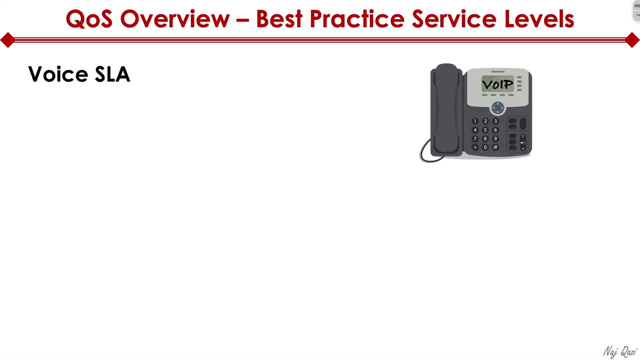 Now let me quickly cover best practice service levels when it comes to voice and video. So for voice over IP, what's the best, SLA or service level agreement, according to Cisco? Cisco says, as long as the delay- one way delay- is 150 milliseconds or less, if the jitter is 30 milliseconds or less. 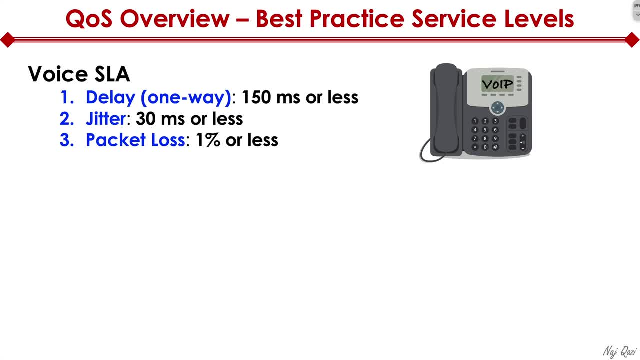 and if the packet loss is 1% or less, then that's considered a good quality voice service level agreement or SLA. Now why do we call it an SLA? This is sort of an agreement with the business that the network is going to provide a certain level of quality to certain types of traffic so the business can continue operating smoothly.